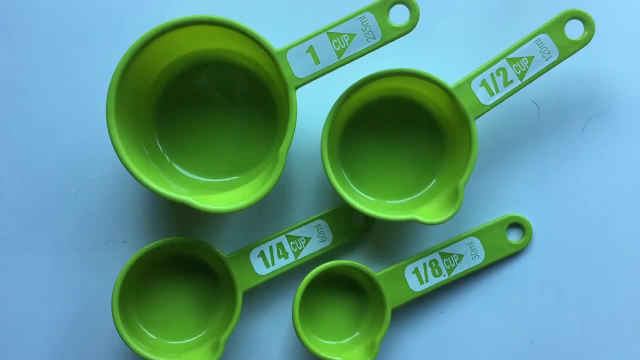 In this video, I want to introduce to you the tools that we use when we're cooking and when we're baking. Now these are called measuring cups. Now we've been talking about fractions in our math unit and I want to show you something: how fractions can be used every day when we're. 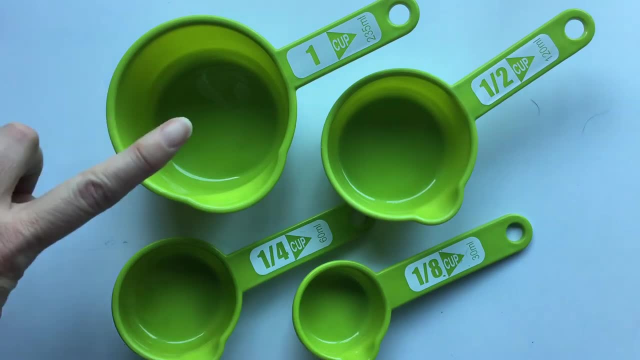 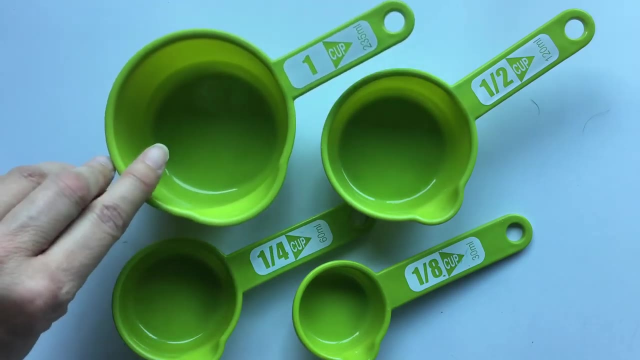 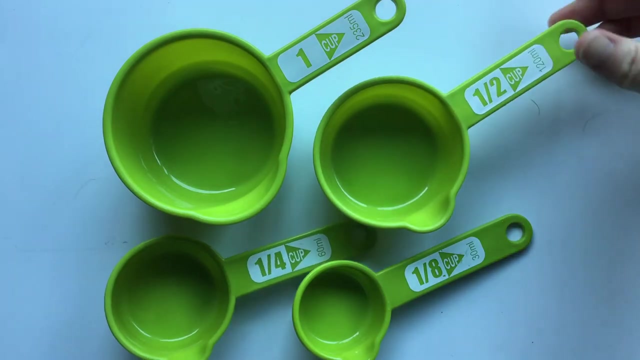 doing our cooking and when we're doing our baking. Now this cup here is called one cup. It is one whole cup, and sometimes you'll see in a recipe it calls for one cup of something okay. Now here's something interesting. This one says one half cup and it is exactly. 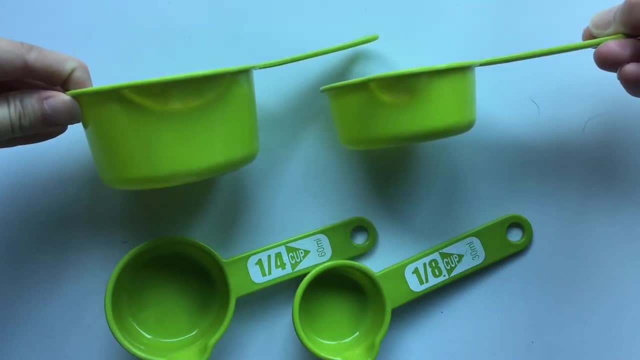 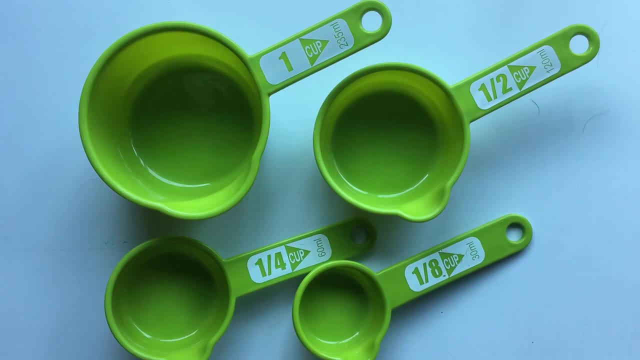 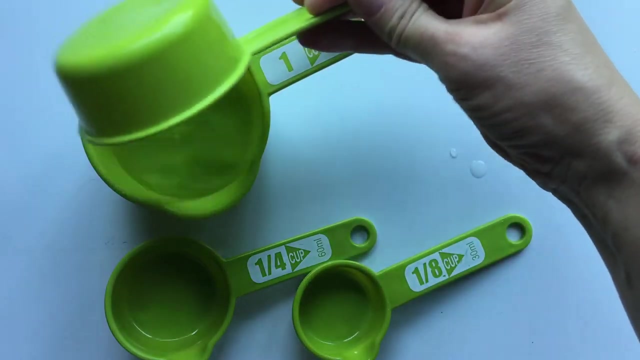 half of this cup. okay, This is the whole. this is the half. okay. And I can demonstrate that to you by pouring some water inside the half cup And then if I pour that water into my one cup, it will fill up exactly one half of the cup. So you can see that one half of the cup has been. 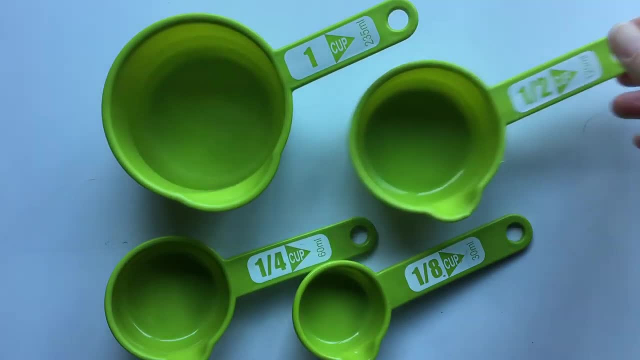 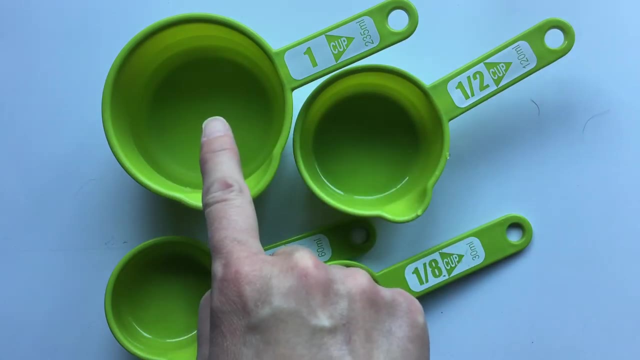 filled. okay, So that's one cup. that's the whole. This is half a cup, which is exactly half of this cup. If I fill this cup, again another half cup and pour it in this cup, what do you think? 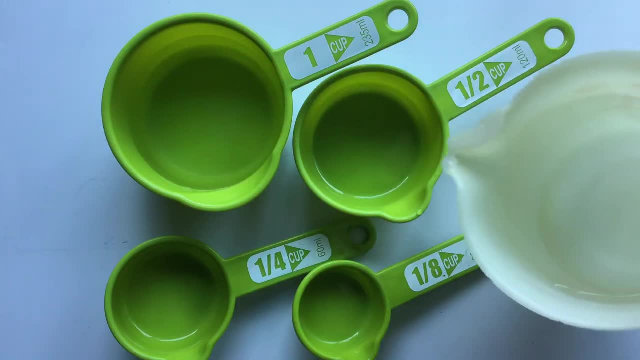 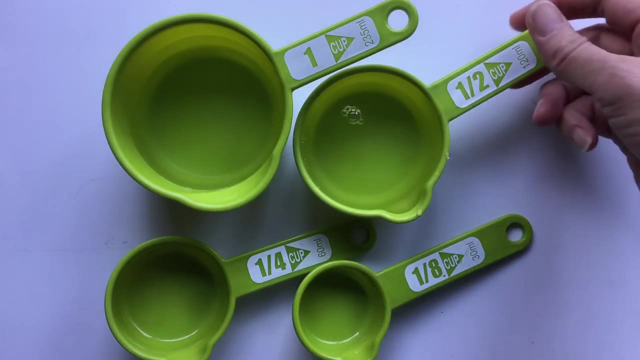 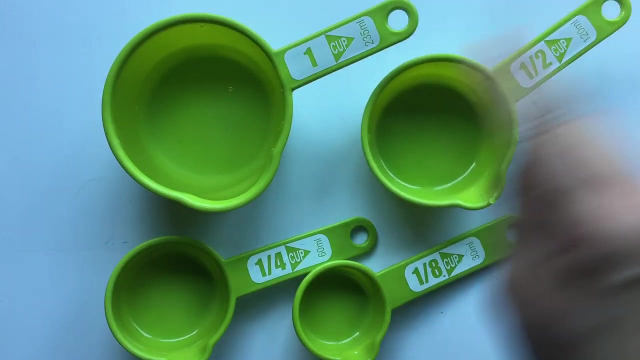 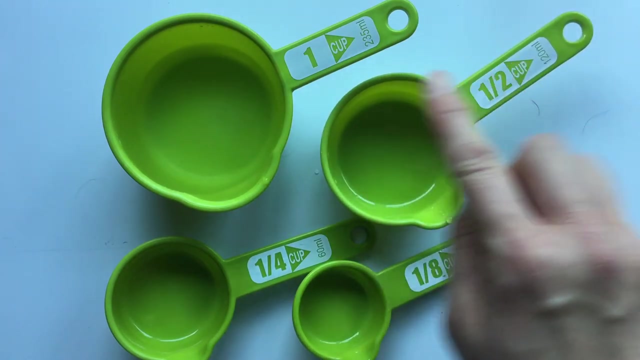 What do you think will happen? Well, let's find out. If I pour two half cups into one whole cup, what happens? I get one whole cup. This cup is now full. My finger goes in the water right away. So two half cups equal one whole cup. So I can say one half plus one half. 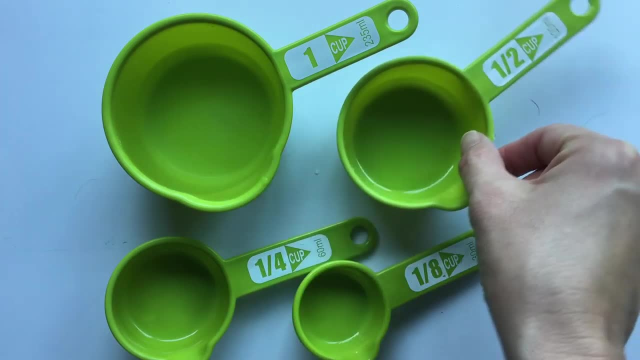 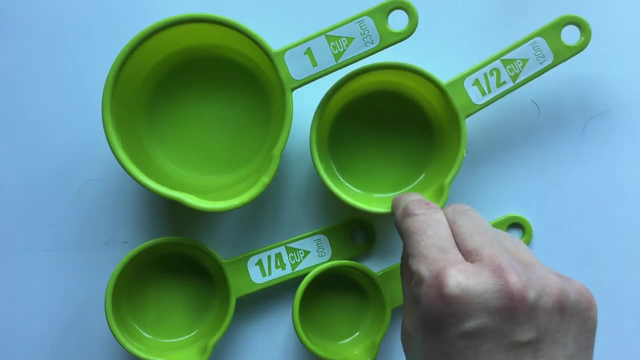 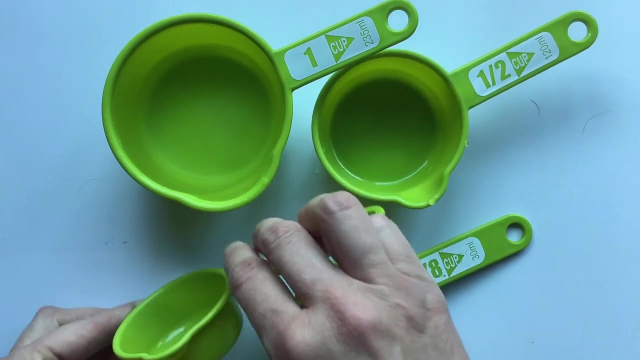 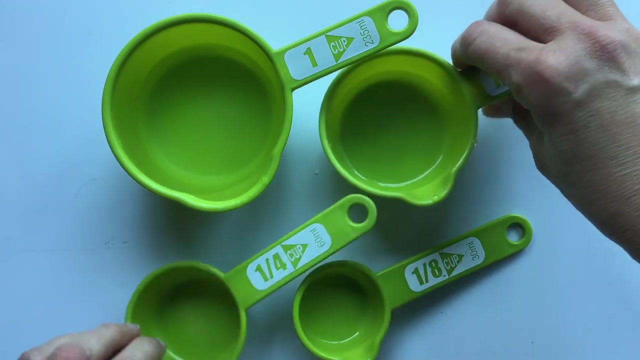 equals one whole. All right, So if you can't find your one cup to do a recipe, you could do two half cups to equal one cup. Now you'll notice here, this is one quarter cup. One quarter cup is exactly half of one half cup. okay, Again, if I were to fill this one up with water.